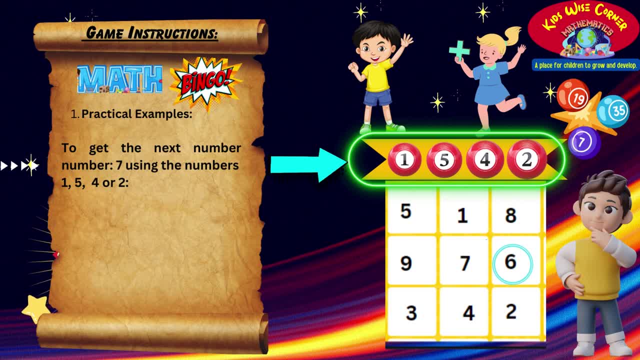 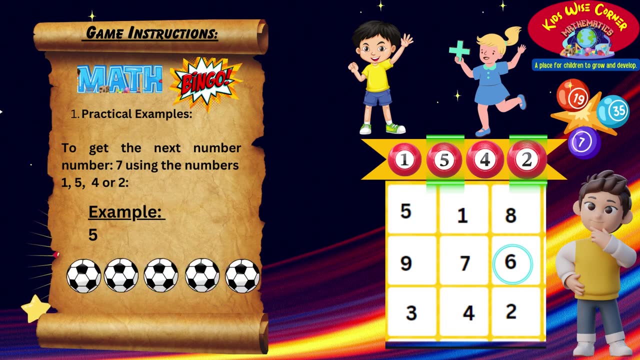 same row as number 6,, which is number 7, using any of the numbers 1,, 5,, 4, or 2,, we need to ask ourselves what sum will give us the number 7? What if we try 5 plus 2?? Do you think 5 plus 2 equals 7?? Yes, 5 plus 2 equals 7.. Let's circle. 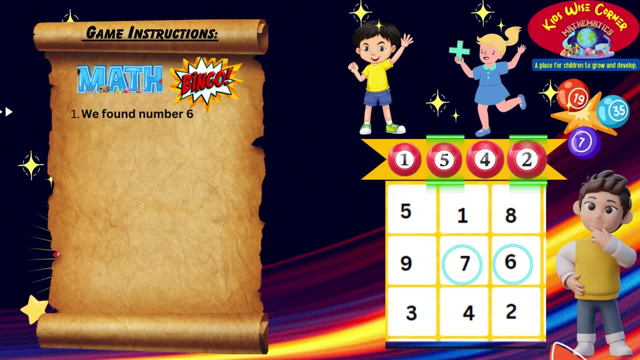 number 7 on the grid. We found number 6.. We found number 7.. To win the game, we need to find the last number in the row, which is number 9.. We need to get the next number, which is number 9,. 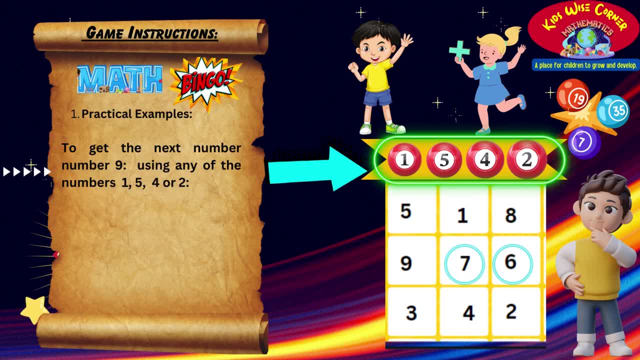 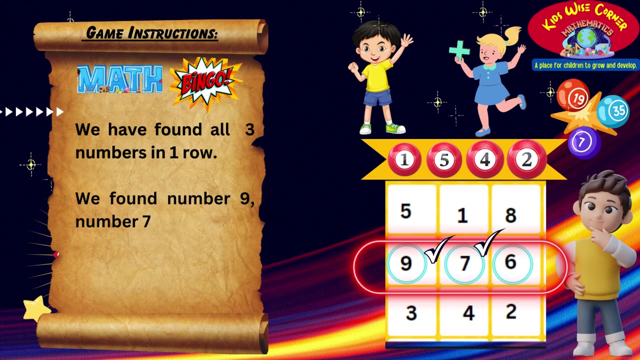 using any of the numbers 1,, 5,, 4, or 2.. Let's try. 5 plus 4 equals 9.. Circle number 9 on the grid. Let's take the numbers we have found. We found number 9.. We found number 7.. We found number 6.. We have found all three numbers in one. 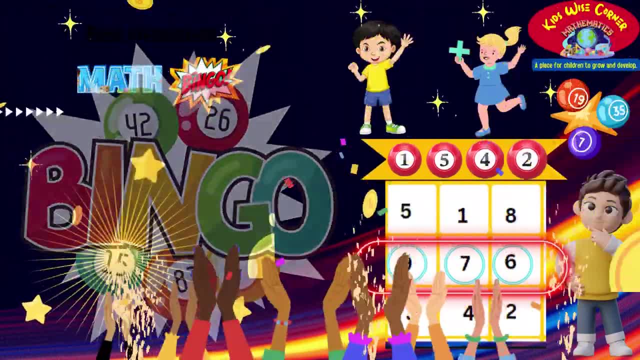 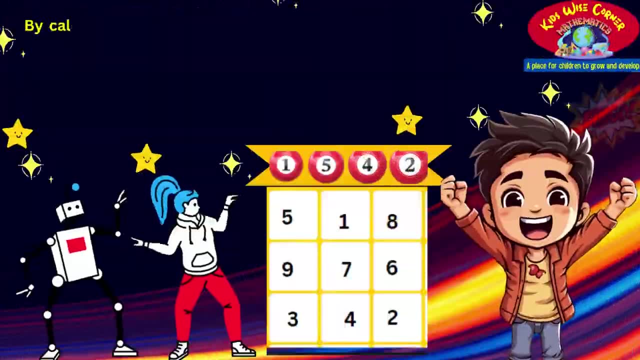 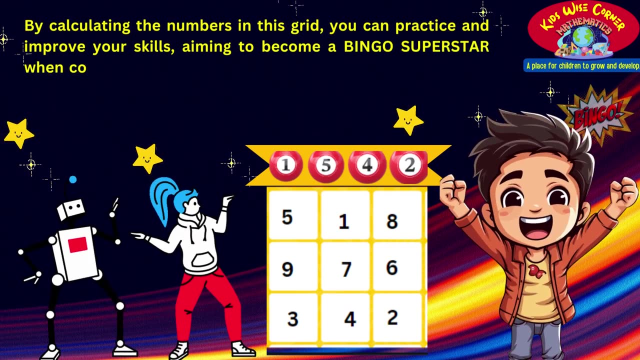 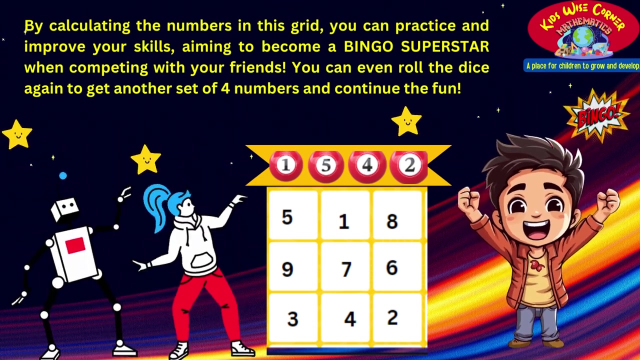 row, You are the bingo champion, Congratulations. By calculating the numbers in this grid, you can practice and improve your skills, Aiming to become a bingo superstar. when competing with your friends, you can even roll the dice again to get another set of four numbers and continue the. 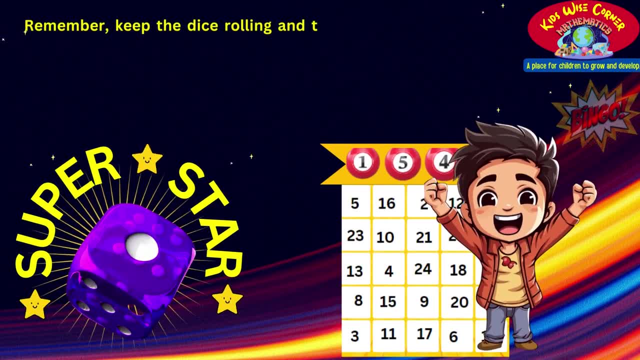 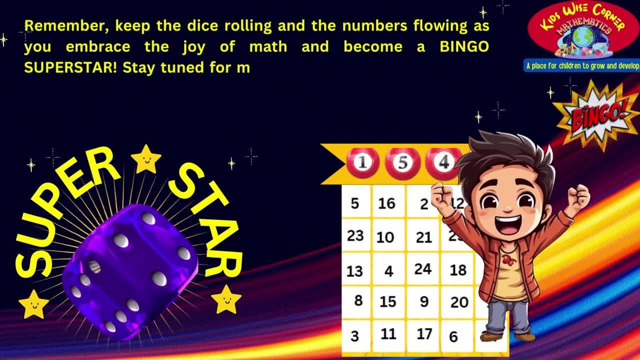 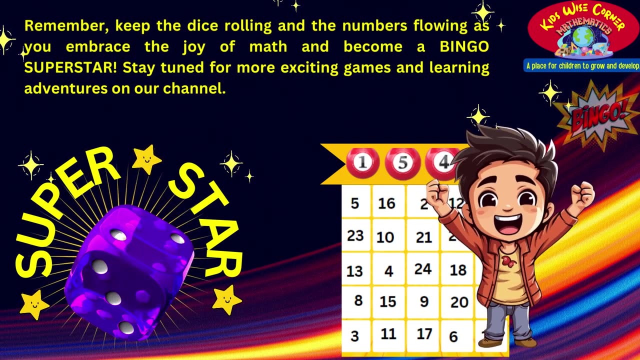 fun. Remember, keep the dice rolling and the numbers flowing as you embrace the joy of math and become a bingo superstar. Stay tuned for more exciting games and learning adventures on our channel. Please look out for my upcoming video on another exciting way to play maths: bingo. 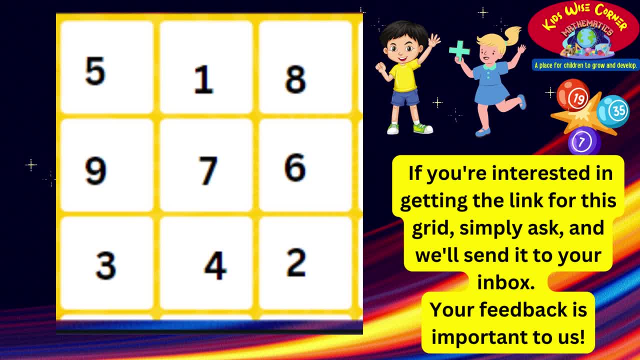 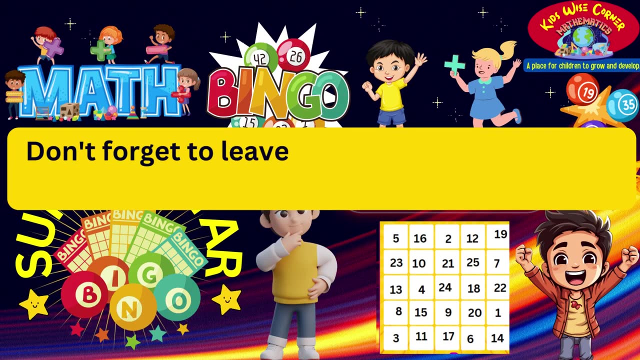 for young kids. Here is the grid for you to use. Thank you for joining us for Math Bingo today. Please leave a comment as to what types of videos you would like to see. If you enjoyed this video, don't forget to like, subscribe and hit the bell icon for notifications on more exciting. 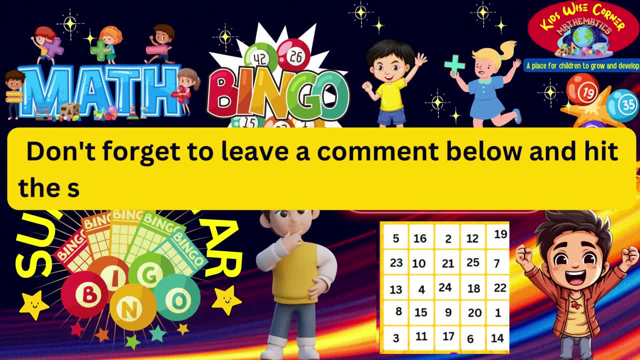 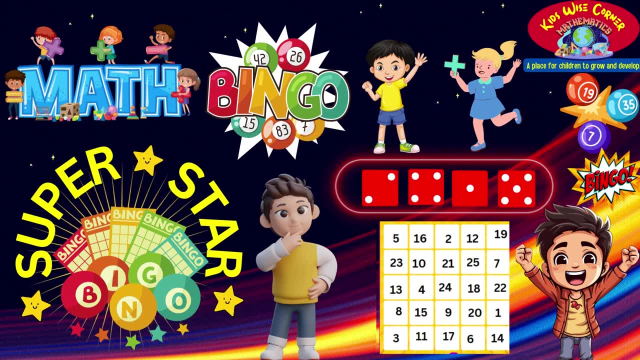 math games and educational content. Until next time, keep playing, keep learning and keep having fun. See you on the next maths adventure. you.